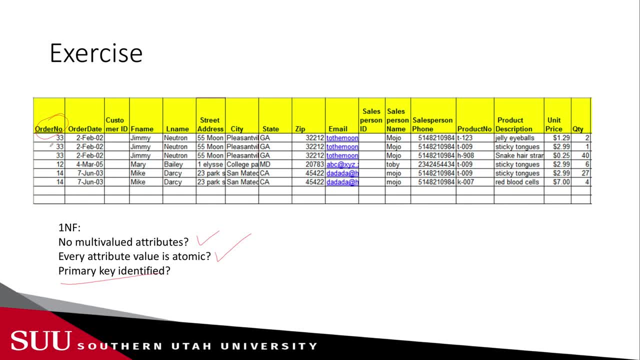 Can we have the order number as primary key? Now we have repeated order number. so obviously not. We have repeated entries in here. repeated entries in here, obviously repeated entries in all of the columns. So we need a composite primary key composed of two or even more attributes. 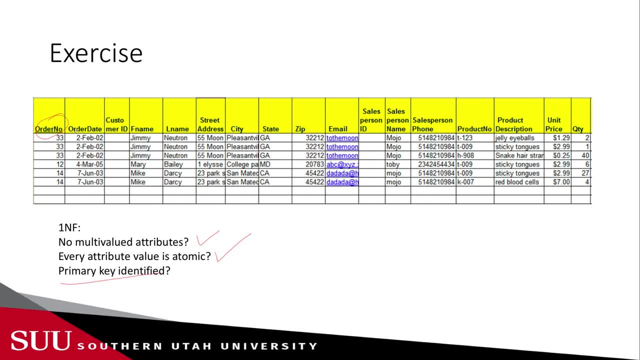 So let's look at combining order number with something else, Since we don't have anything in here: the IDs of the salesperson and the IDs of the customers. let's look at something else. that's an ID. What about product number? Because, again, if we use the salesperson, 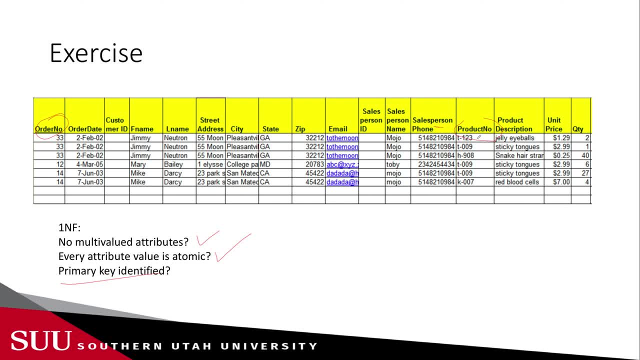 The phone or the customer email is going to be repeated. But now this specific number: is it repeated for the same order number? The answer is no. Is this repeated for the same order number? The answer is no. Is this repeated? No. 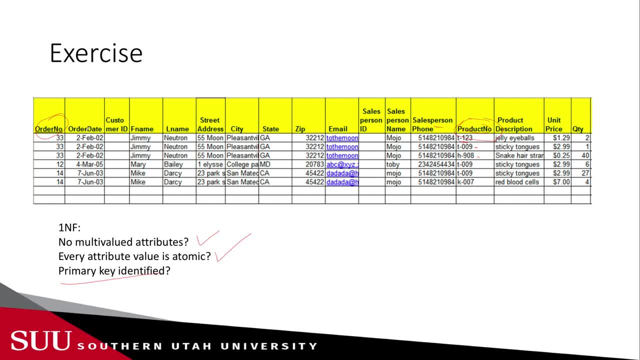 So if we combine product number with order number, can we get a unique combination in every single row of this Excel sheet? The answer is yes. Okay, So we have defined our key as a composite key of order number and product number. Does this take me to the first normal form? 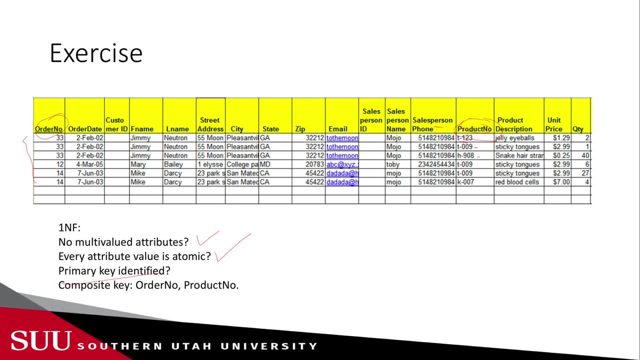 The answer is yes, Because the steps I need in the first normal form is to define my key and to take out any multi-valid attributes. So what is going to be my table in the first normal form? The answer is this: is the table. 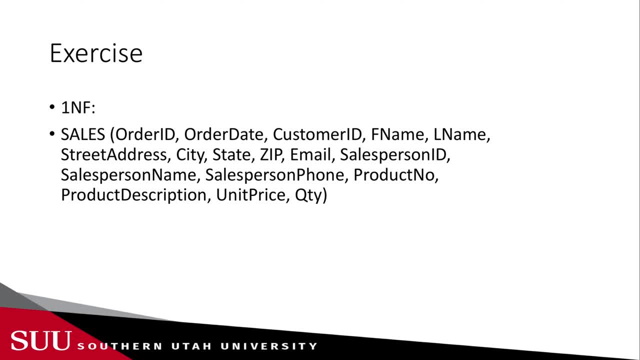 We will call it sales, We will have all the columns in there, But we need to make sure that we highlight the order ID and the product number as our key. So these need to have underlines underneath them, And this is my first normal form. 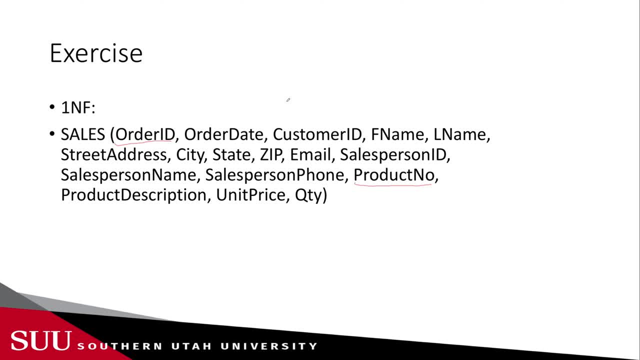 Now, when I'm in the first normal form, what's going to be next? Do I just leave it like this? The answer is we need to take it to the second normal form. Okay, Okay, So I'm going to take it to the second normal form. 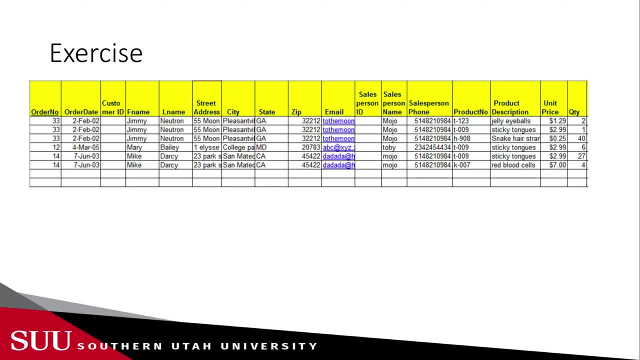 Now this is my table in the first normal form and I have the keys highlighted. So I have underlined order number and I need to underline product number. So these are underlined now and this is in first normal form. Now to get it into the second normal form, we will need to get rid of all of the partial. 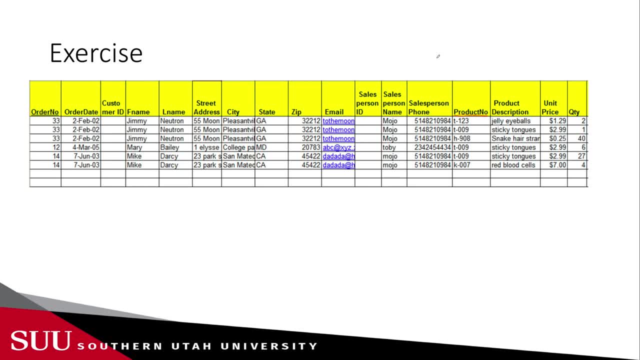 dependencies. First of all, let's see, First of all, let's check up for all the dependencies we can see. in this case, Let's check first for full dependencies. Do we have any full dependency? Remember, a full dependency is when any attribute relies on the full key. 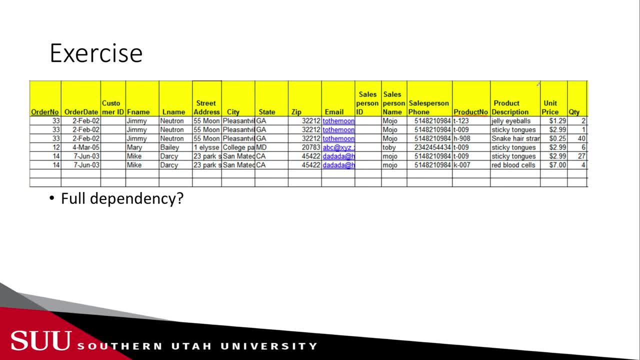 So what is going to rely on order number combined with product number? It is the quantity, So we have a full dependency for the quantity on product number. Okay, So we have a full dependency for the quantity on product number. So this is one dependency which is a full dependency. 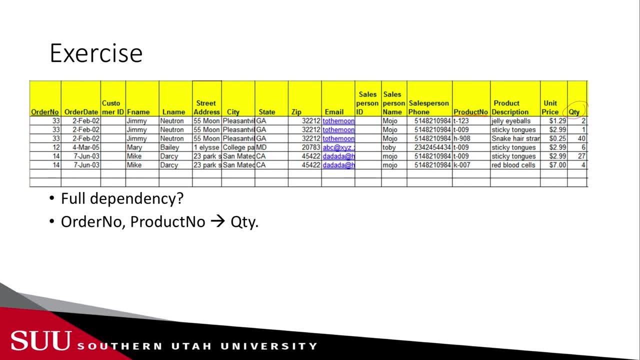 Do we have any other full dependencies? The answer is no. Do we have any partial dependencies? So partial dependency is when something relies on part of the key. The answer is yes, We have a partial dependency on the order number. So the order number in this specific table. 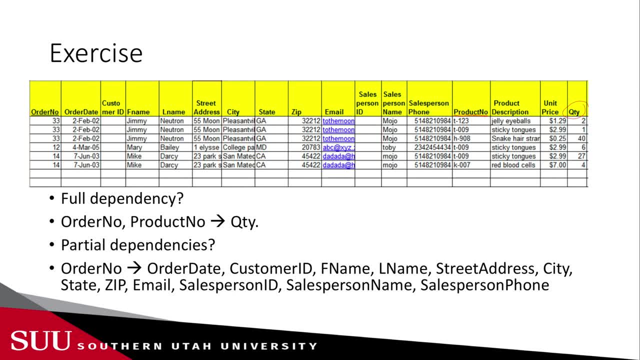 Now, remember that we are dealing with what we currently have. We don't. We don't jump in advance and say this is going to be the key later on. No, We just deal with what we currently have in this case. Now, in this case, we have the order number determining the order date. customer ID with. 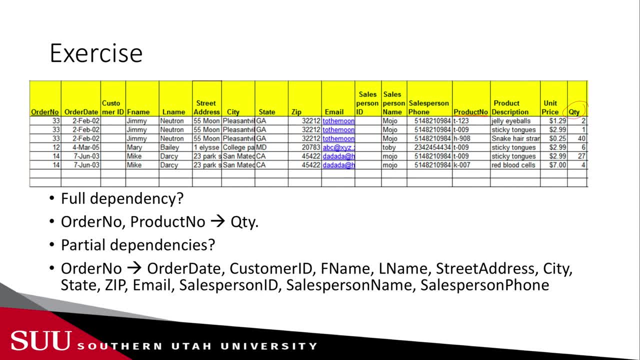 the first name, last name and the address and the customer information. The order number is going to also tell me who is the salesperson for that order, containing the ID and the name and the phone. So this is one partial dependency. Okay, Do we have another partial dependency, something on the product number? 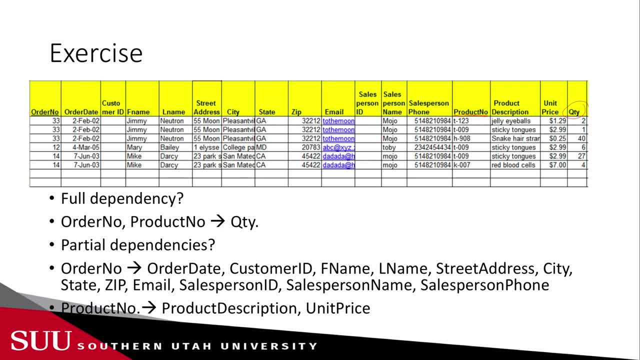 The answer is yes. The product number is going to tell me the product description and the unit price for that product. Now, what do I need to do with those dependencies? I need to get them out of the table. How do we do this? 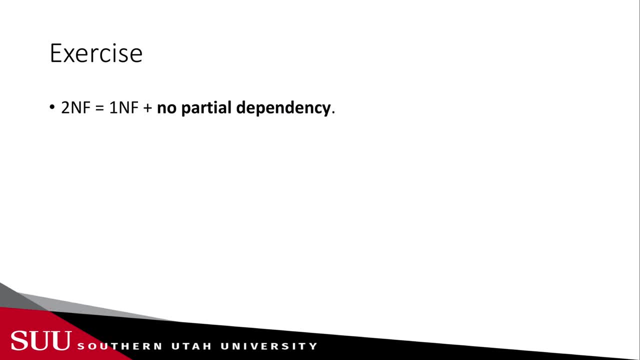 By separating them into their own tables. So to go to the second normal form, again, we said it is the first normal form but we need to remove the partial dependencies And we will have the sales table containing order number, product number and quantity. This is one full dependency. 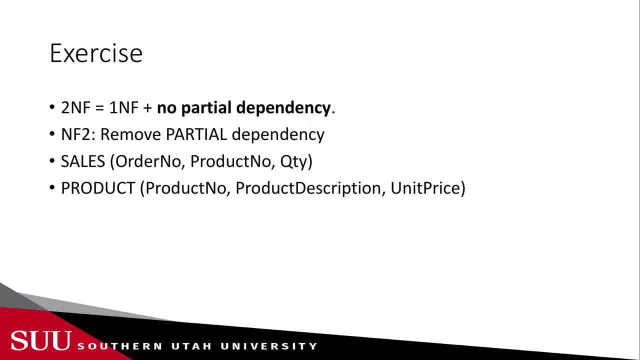 We will convert the partial dependencies to full dependencies by saying: product is going to have product number, product description and unit price. This is again a full dependency. Then again, order is going to contain the rest of the attributes, And this is a full dependency. 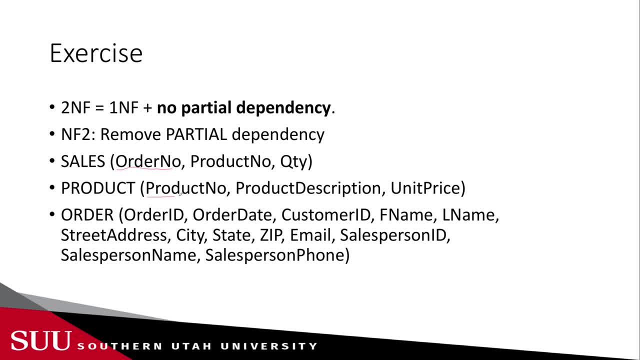 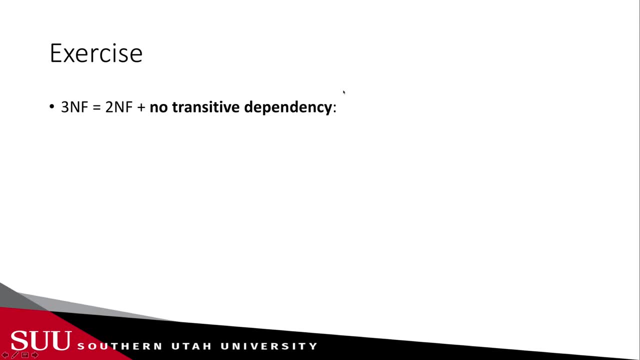 Okay, So we need to remove the partial dependencies And we need not to forget to underline our keys in this case, which is going to help me in the next step. So what is the next step? My next step is to jump to the third normal form. 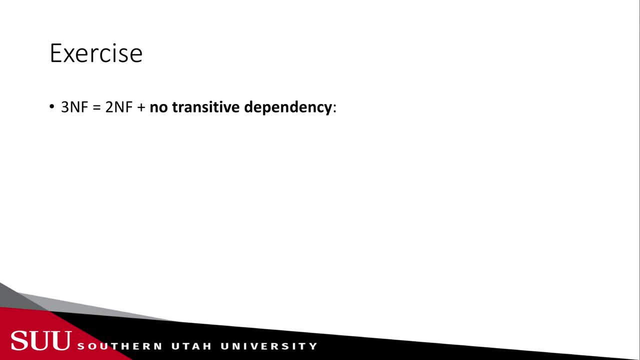 And the third normal form is nothing but the second normal form with transitive dependencies removed. So let's list our tables first And remember that the first normal form is the second normal form. Remember that my keys are: order number for this table, product number for this table. 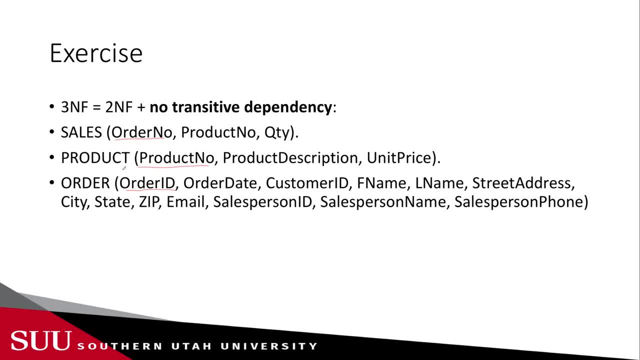 and order ID for this table. Now, do I have any transitive dependencies? Remember, a transitive dependency is when a non-key attribute depends on another non-key attribute. So let's look in this table: Do we have something that's a non-key attribute relying on a non-key attribute? 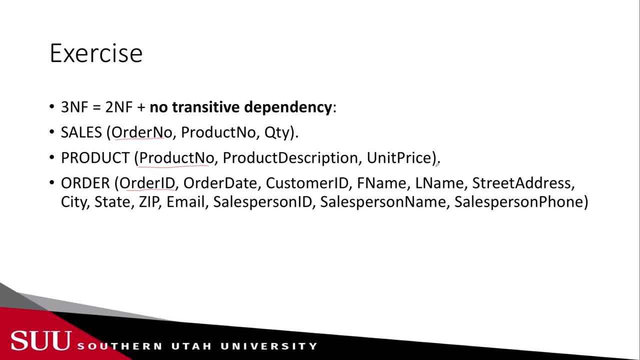 The answer is no. Do we have something like that in this table? The answer is no, Do we have something like that in this table? Now look at the customer ID. Isn't this going to tell me who is the customer name, or first name, last name, address and? 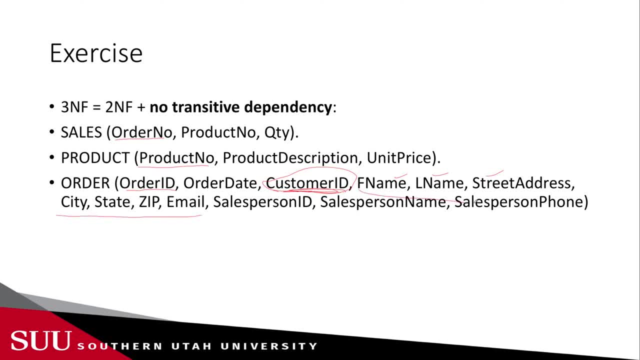 all this information, So all of those information here Are going to be determined by the customer ID. So this is one of the transitive dependencies that I have in this table. Now, if we look closely, do we have any other transitive dependency? 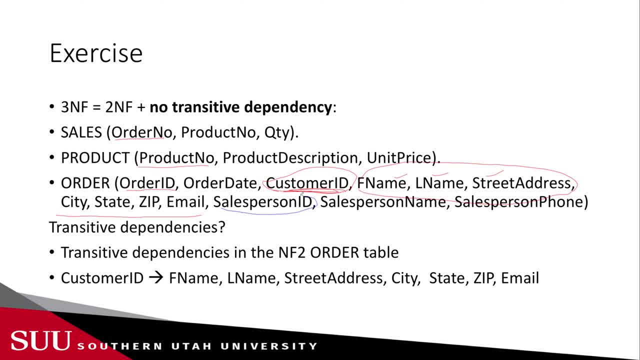 What about salesperson ID? Does this tell me anything? Now, the salesperson ID is what's going to determine the name and the phone of the salesperson. So that tells me that I have another transitive dependency. Now the rule says I will need to take these out, create their own tables. 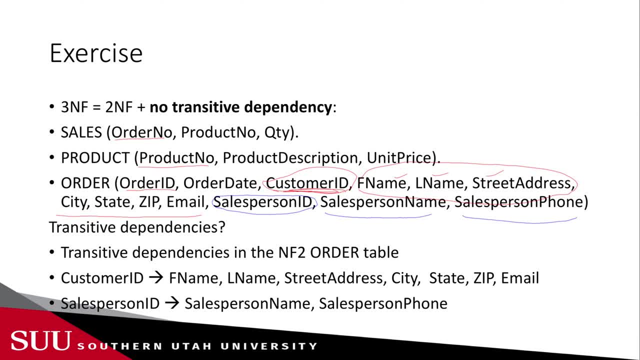 Customer ID is going to be a key for the customer table, Salesperson ID is going to be a key for the salesperson table, But then I need to keep customer ID and salesperson ID in the order table as foreign keys. This is the rule of how to get rid of transitive dependencies. 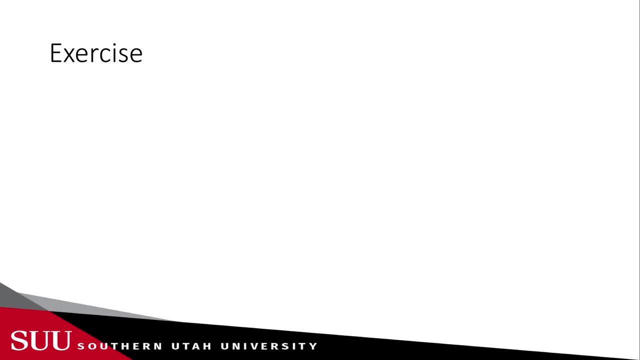 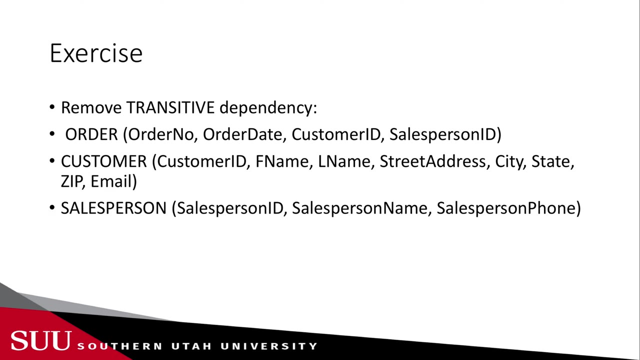 So my list of tables is going to be the following. I will have order number, order date, customer ID and salesperson ID in the order table. Customer table is going to have customer ID and all of the customer information. Salesperson is going to have the salesperson ID and all of the salesperson information. 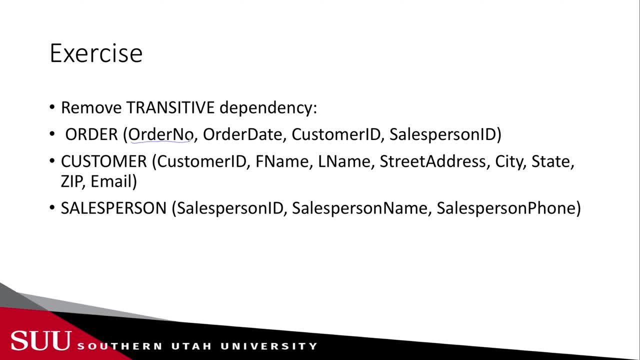 Now, what about the customer table? What are the keys? We know for a fact that this is a primary key. This is what we created as a primary key And this is what we created as a primary key, But the rule says we need to keep these as foreign keys, preferring or referencing the 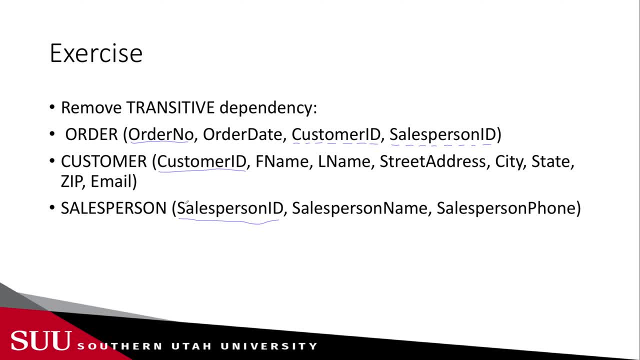 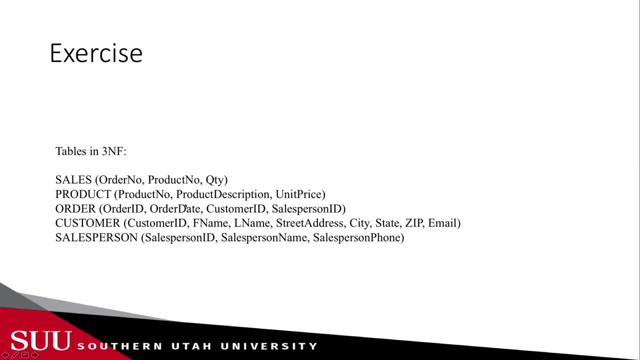 tables below. Now the only thing left is to combine all of those tables and to list them all together as follows. Now, these are going to be my tables, And I just need to highlight my keys in here. So the serials is going to have this as a key. 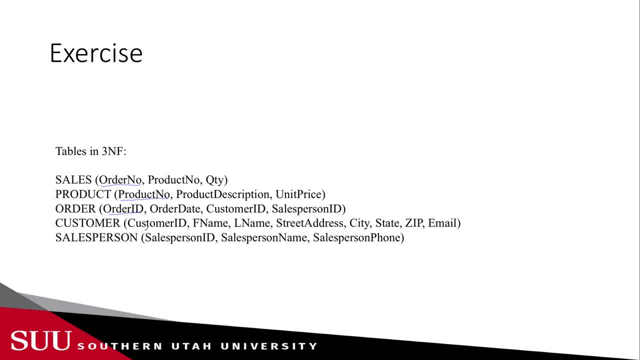 This is going to be the key here. This is going to be the key, And this is going to be the key, And this is going to be the key. Now, let's not forget the foreign keys. This is going to be a foreign key. 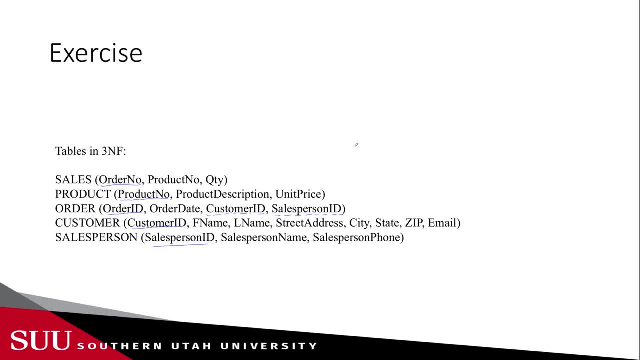 And this is going to be a foreign key. Now, do you see any differences? No, So do you see how we moved from a traditional file processing system, which is an Excel sheet, into a full database approach? We have the full list of tables without going through the requirement collection, without